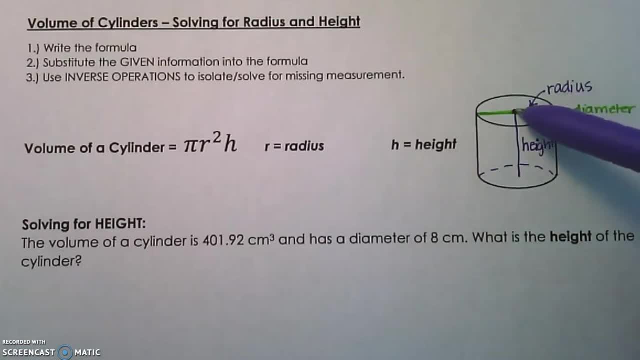 So, looking at this picture here, you can see that the purple line that goes from the center of the circle to the outside of the circle, that's called our radius, And then the height is going to be from the center of one of the circle bases down to the center of the opposite. 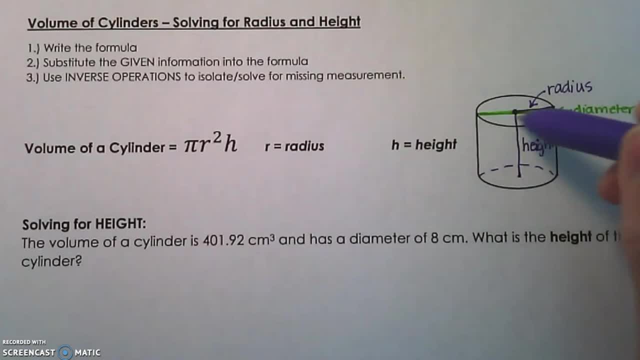 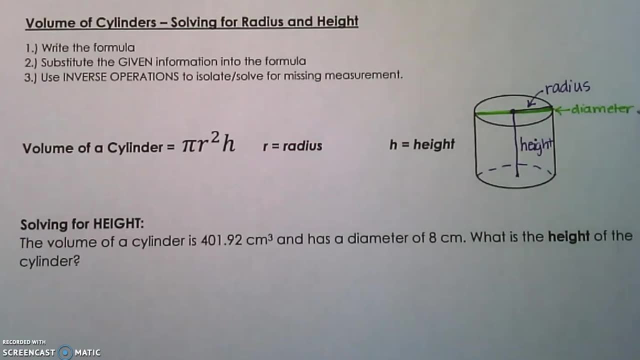 circle base. that is your height measurement. And then the green line here that goes all the way across through the center of the circle from one side to the other. that's called the diameter, And the diameter is twice the distance of the radius. So we're going to 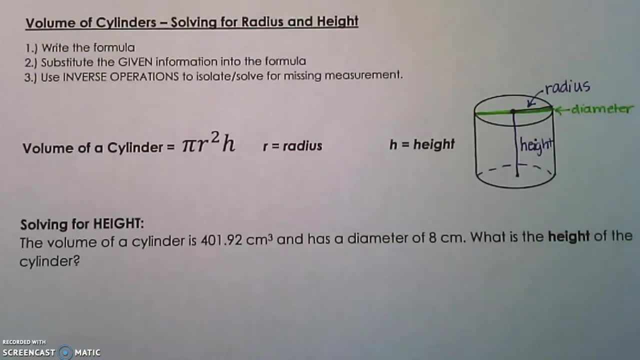 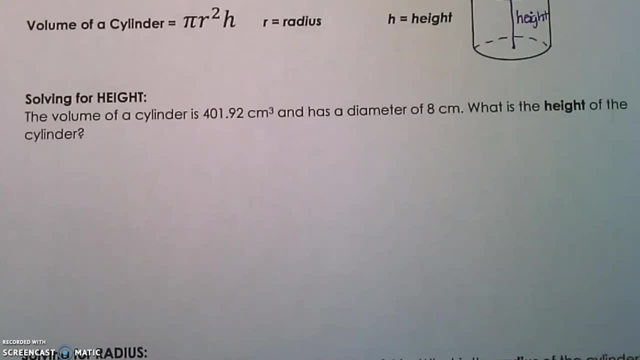 in one of our examples we're going to be using diameter and we'll talk about how to get radius from that measurement. So let's look at the first example, solving for height, Given, the volume of the cylinder is 401.92 cubic centimeters with a diameter of eight. 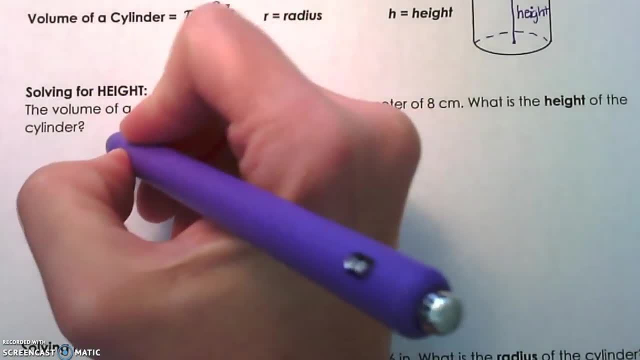 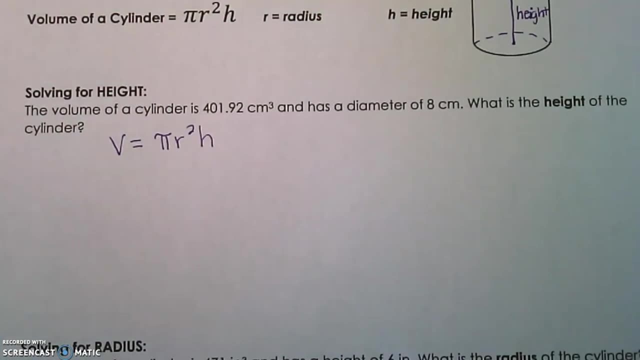 centimeters, what is the height of the cylinder. So let's first write down the volume, pi r squared times height, write down our volume formula And we're now, we're going to substitute the given information in, So we know that the volume is 401.92.. So 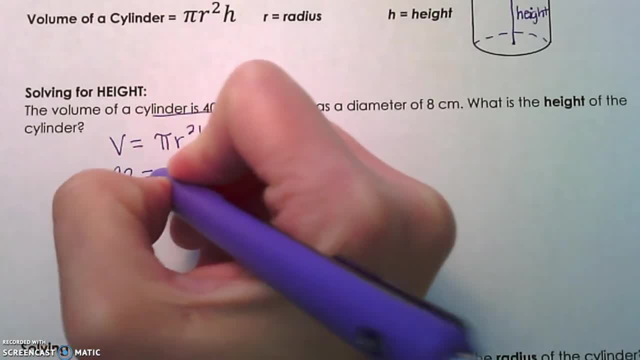 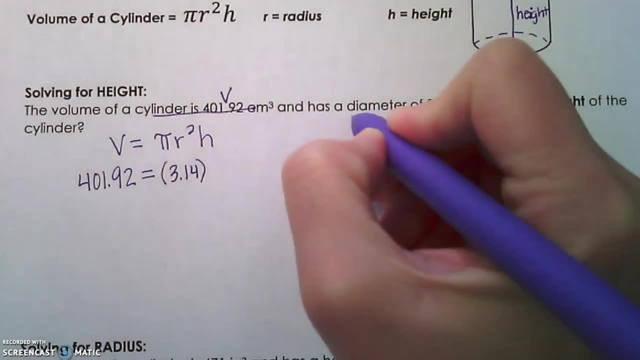 we're going to sub that in for v in the formula. We're going to use 3.14 for pi in all of our examples, times the radius squared. Now we're given diameter is eight. So that means the radius is going to be half of that which is four. So we're going to use the radius. 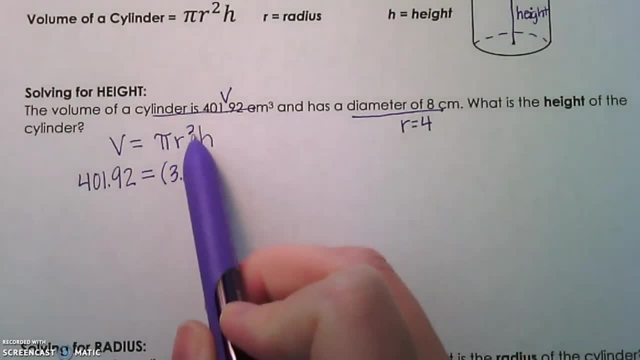 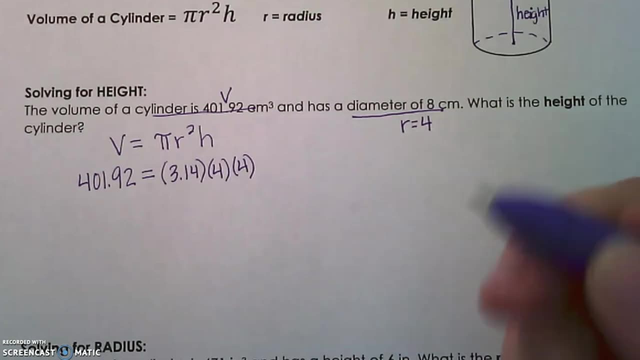 squared. We're going to use that measurement because that's what our formula is calling for And we need to square four, So I'm going to write four as a factor twice. I feel like that helps. remember that we're multiplying the factor twice instead of multiplying by. 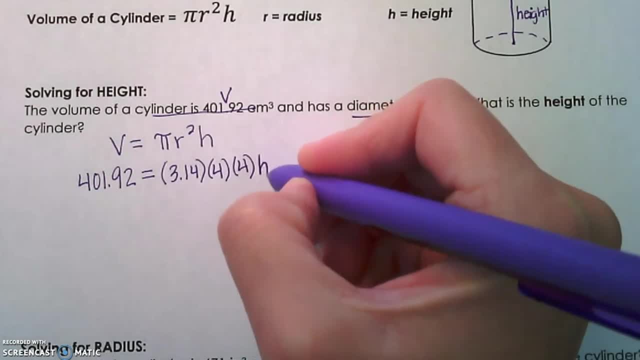 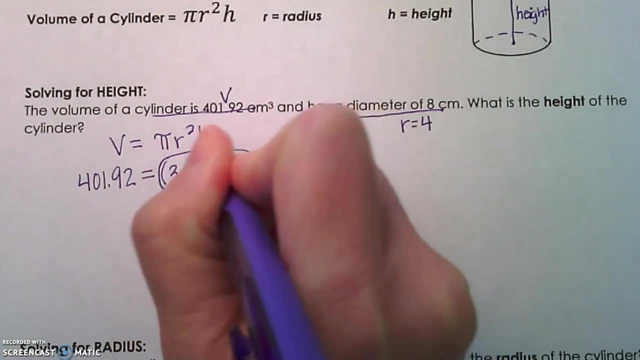 two. That's your difference there. And then we're looking for height. So we're just going to write H, because we don't know what that number is. All right, So our next step is going to be to go ahead and multiply pi times radius squared with our calculators. So when? 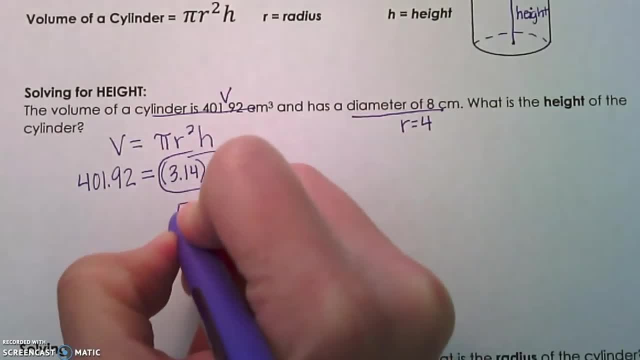 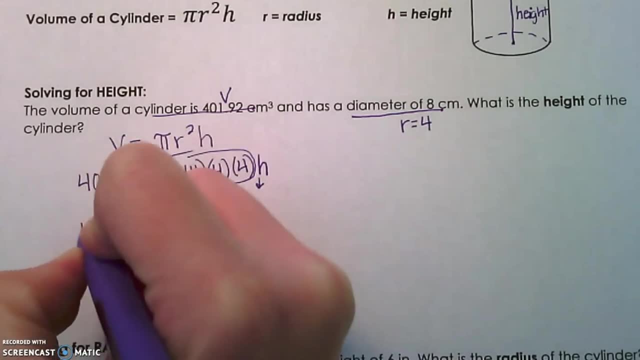 we plug those numbers into our calculator, we get 50.24.. Times H is still going to come down because we have not done anything with that variable yet. We're just one step closer to solving for it. Now we're going to divide both sides. 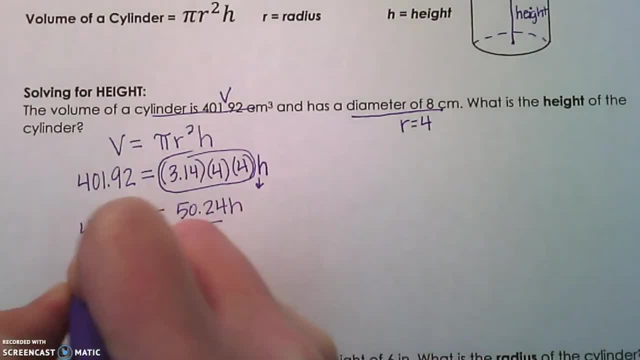 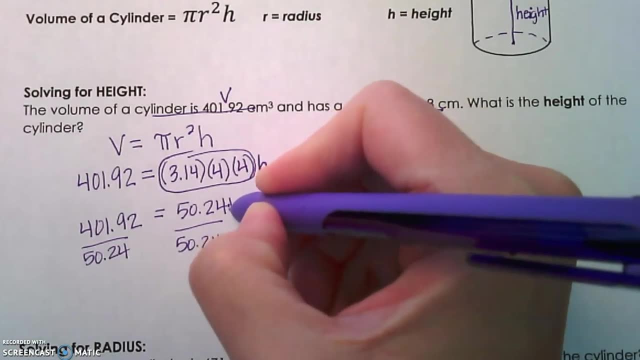 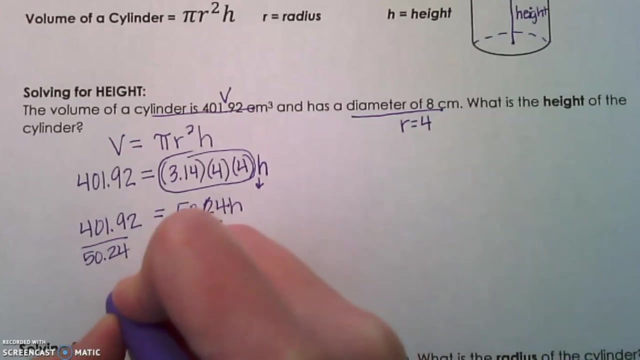 by 50.24.. That's our inverse operation, right? Because 50.24 times height, the inverse of multiplying would be dividing. Okay, So those 50.24s are going to cancel out and we get that our height is equal to eight.